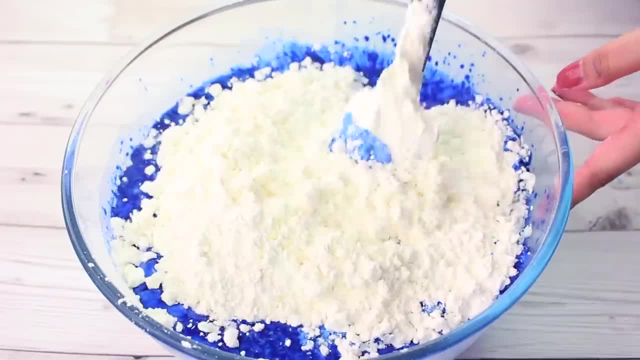 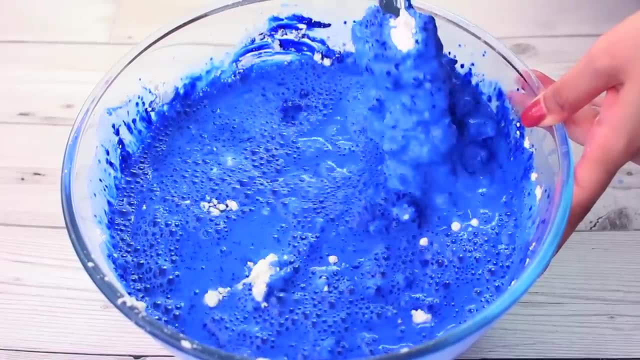 it just dissolves. but the more corn starch you add, the more thick the mixture will become and it will become a lot harder. So what I recommend doing is just pushing the corn starch under and then, at a later stage, just going in with your hands and breaking up all the lumps. But you just want to keep getting the corn starch under and trying to get it to be a little bit thicker. So I'm going to add a little bit of corn starch and then I'm going to add the rest of the corn starch, and then I'm going to add the rest of the corn starch. 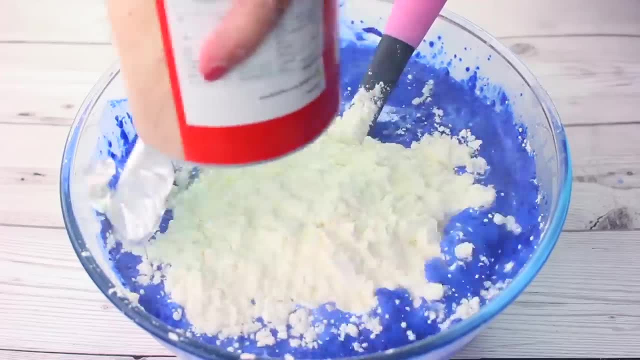 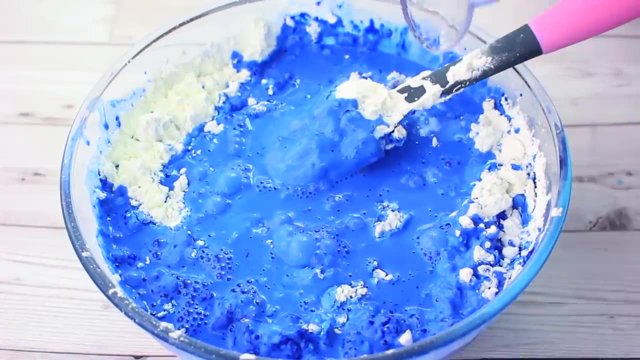 After adding in the second batch. I do recommend just taking it a bit slower because otherwise the mixture can get really thick like this, because I added a bit too much corn starch and I needed to go in and start over and add some more water And I needed to go in and 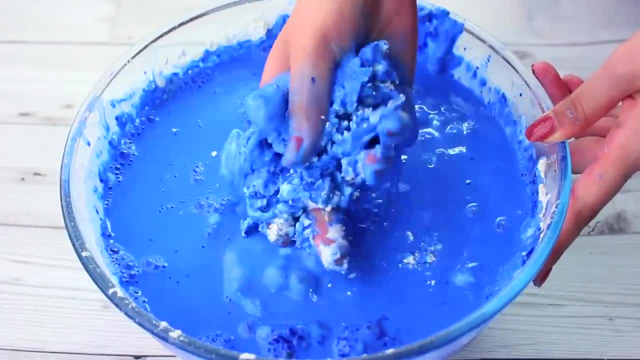 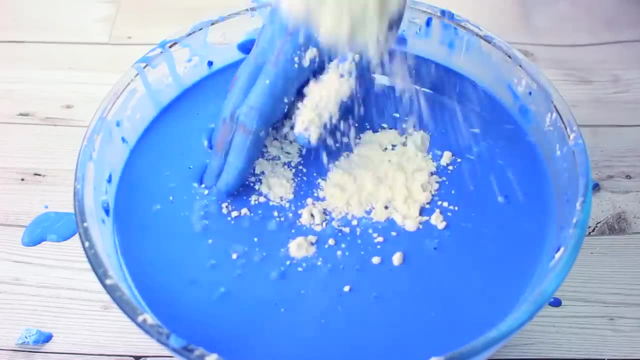 break it up with my hand, which became quite messy, but again, this just helps the texture get a bit better and you just want to keep adding corn starch again until it becomes thick And, as you can see there it was a bit too thin, so I added a tiny bit more and, as 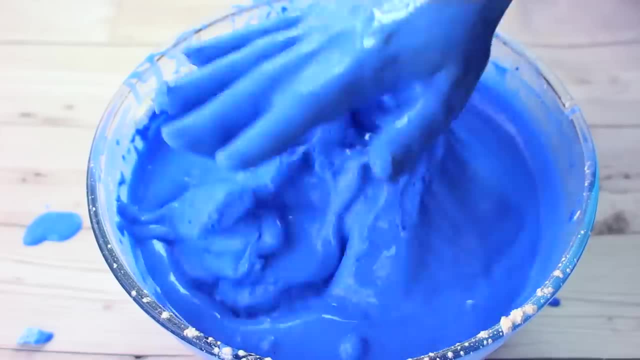 you can see, it's made all of the difference. The tiniest bit makes it super thick and the thickest bit makes it super thick. so don't rush this method and you're going to be left with a really cool slime And I don't really recommend eating lots of this. normally it's. 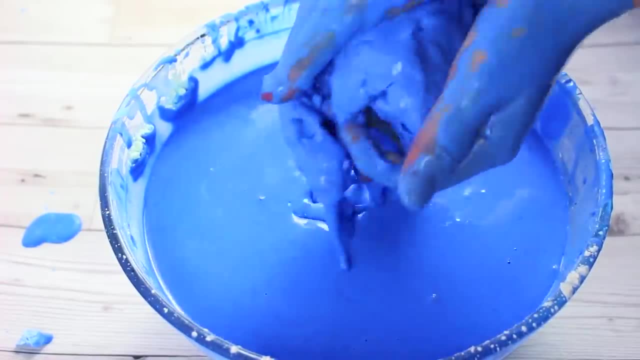 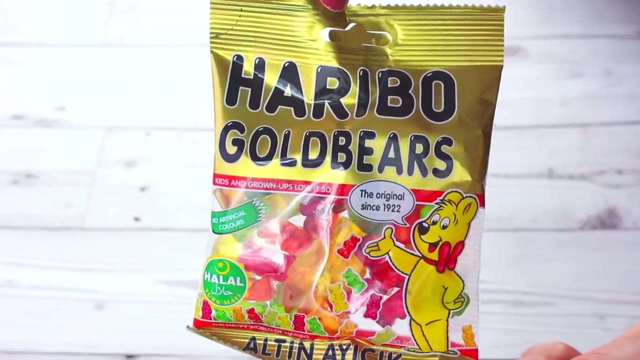 used to like thicken up gravy, but you can have like a teaspoon worth. I just wouldn't recommend having the whole bowl. Last but not least, we have a slime that really surprised me and was so stretchy even when it cooled down, And this is made out of haribo gummy bears and I just added a whole pack. 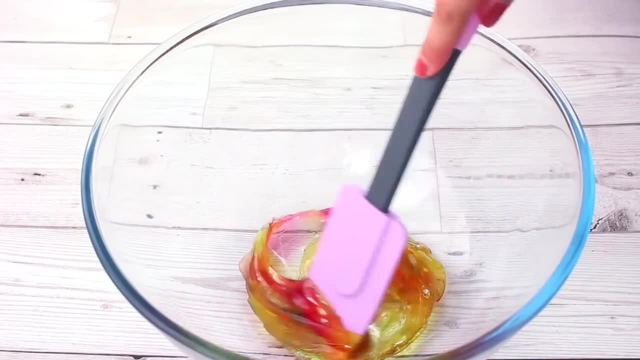 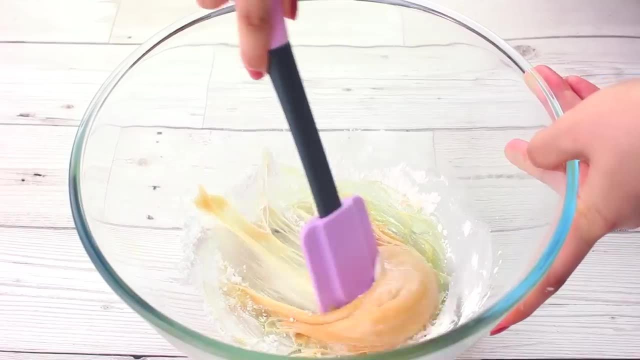 of this, and this really didn't take a long time to melt- I think it was about 10-15 seconds in the microwave on top heat. The mixture was so sticky, so I went ahead and added a whole tablespoon of icing sugar to start off with, And the mixture kind of looked like caramel. 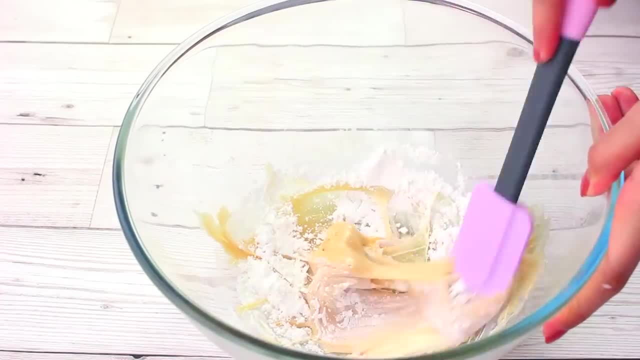 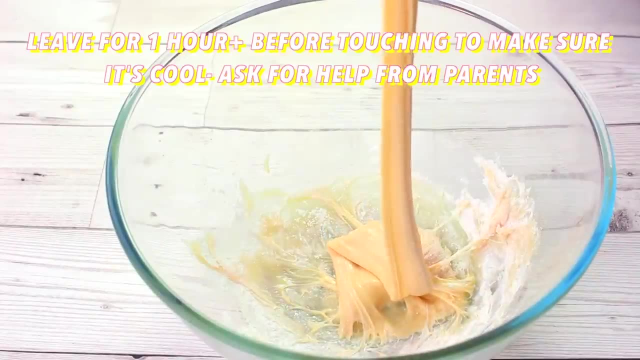 it was so sticky and it was just such a nice texture and it wasn't an ugly colour either, which I was really surprised with, because all of the colours were mixed together. So I just kept adding my icing sugar really gradually, and eventually it was losing its stick a bit. 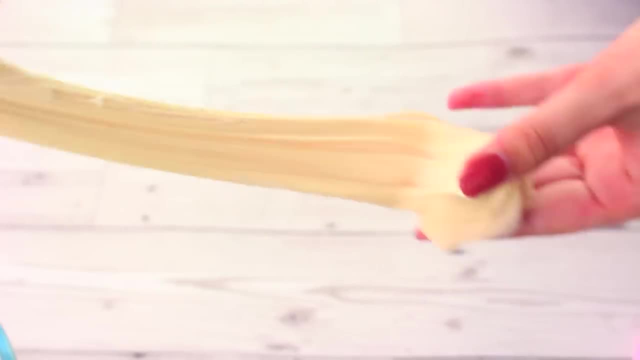 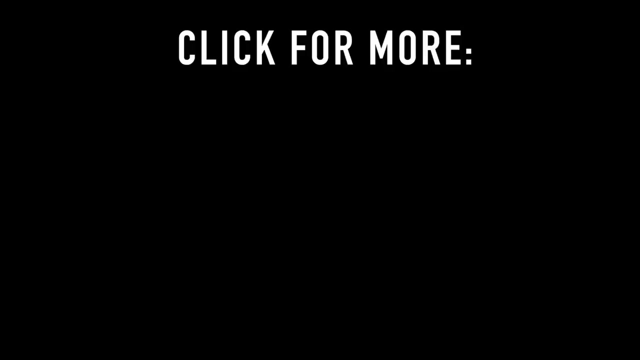 I was really worried that when I started playing with it it would become like a dough, so I started adding it gradually with my hands and playing with it, and it became such a nice texture and was so, so stretchy. I really hope that you enjoyed this video and if you did, don't. forget to give it a thumbs up and I'll see you next week. Subtitles by the Amaraorg community.